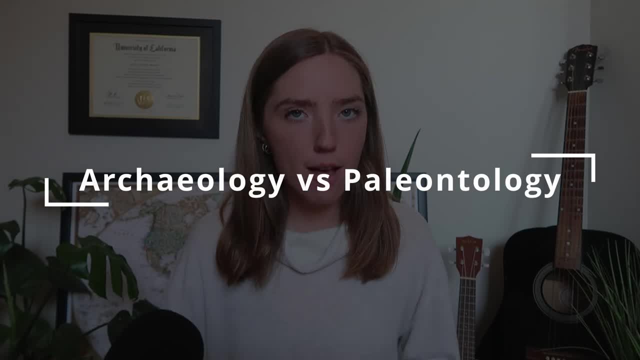 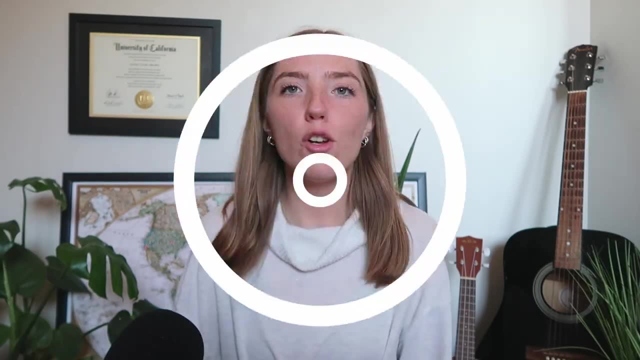 between archaeology and paleontology because they sound pretty similar, but they are in fact very different things, So let's just get into it. So in this video today, we're going to be starting out with those basic definitions that you're going to find on Google. Then we're going 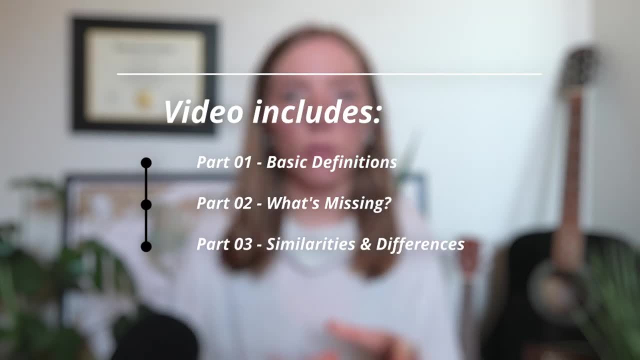 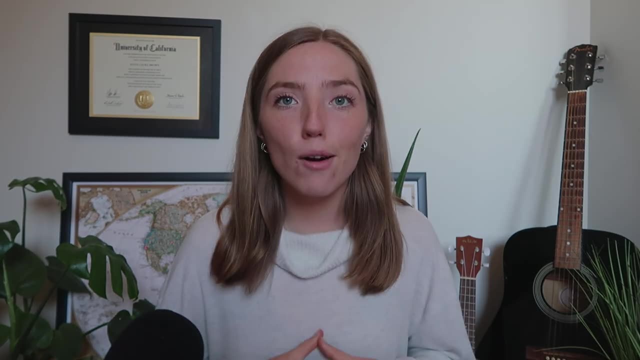 to dive into what's missing from those definitions, And then we're going to close this whole thing out by talking about the differences between the two fields and the similarities. So let's start out with archaeology. Now, if you look up archaeology- the basic definition that Google's going to give- 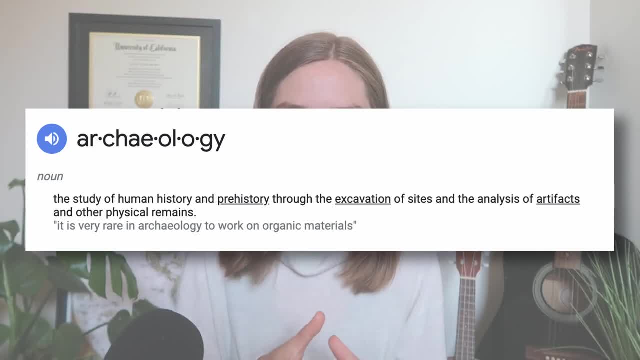 you is the study of human history and the history of the world. So if you look up archaeology, you'll find prehistory through the excavation of sites and the analysis of artifacts and other physical remains. So this might be exactly what you're expecting. I'm not sure, but I want to. 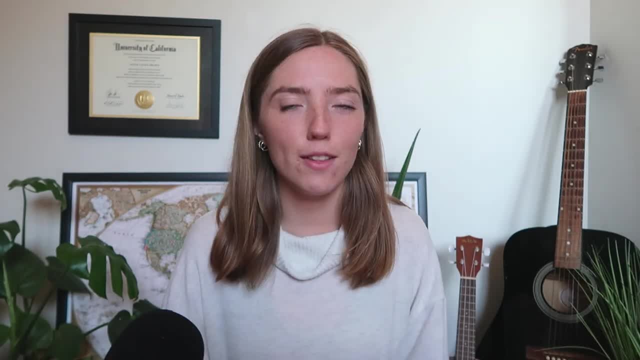 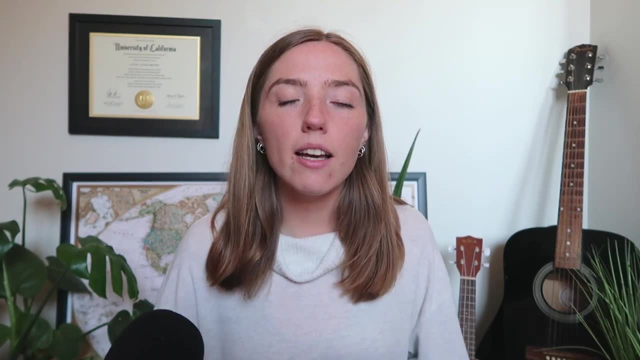 draw your attention to one little word in this definition that kind of changes everything, That word being human. Archaeology, like it says, here is the study of human history. okay, through the things that we excavate. That's what I want you to take away. 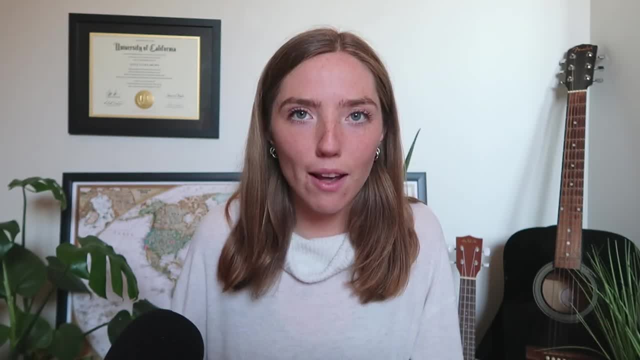 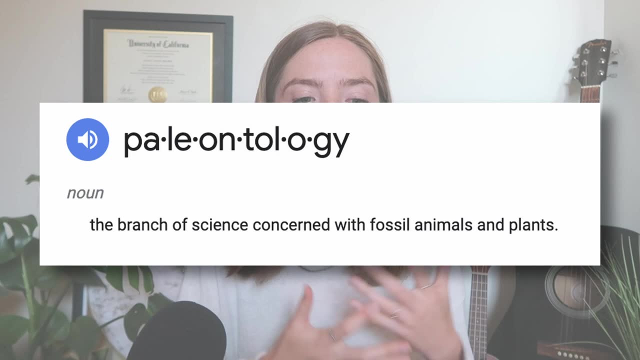 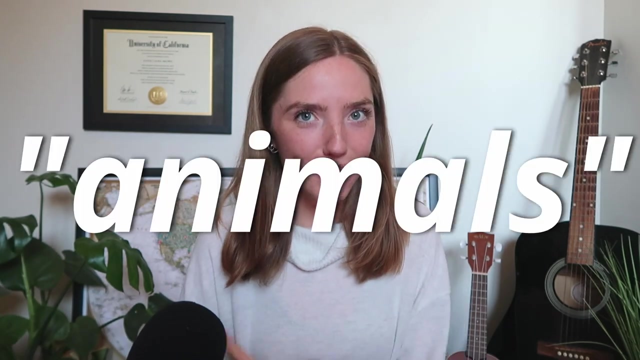 From this definition as we now transition into the next definition, which is paleontology. So when you look that up, you're going to get this: The branch of science concerned with fossil animals and plants. Okay, take a guess on what the keywords in here are: Animals and plants- Those 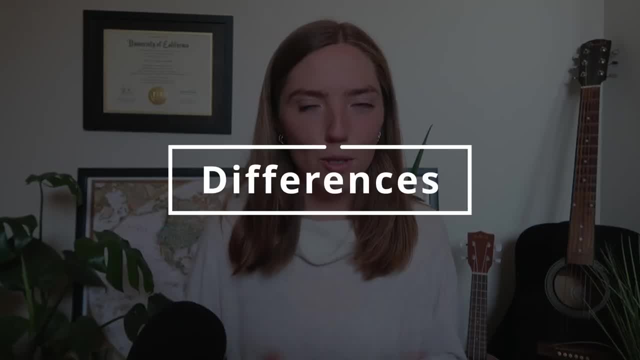 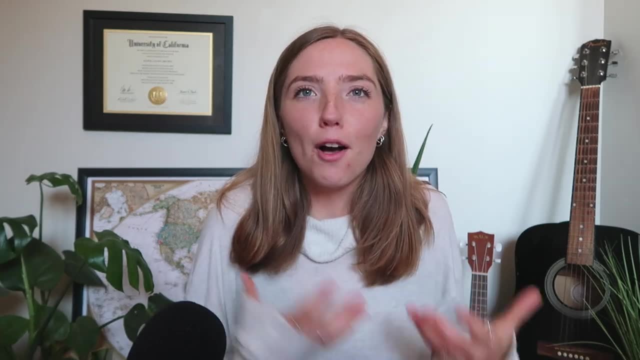 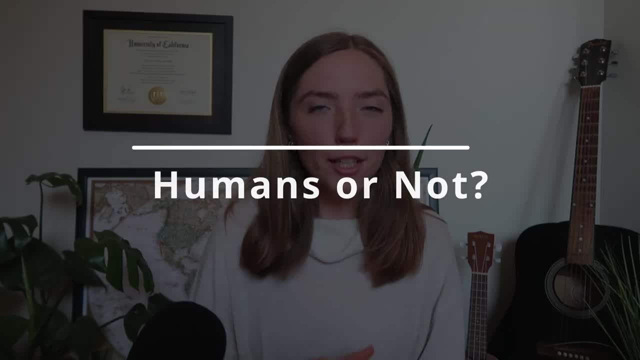 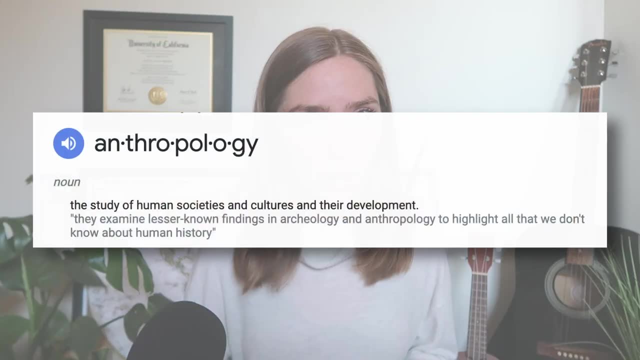 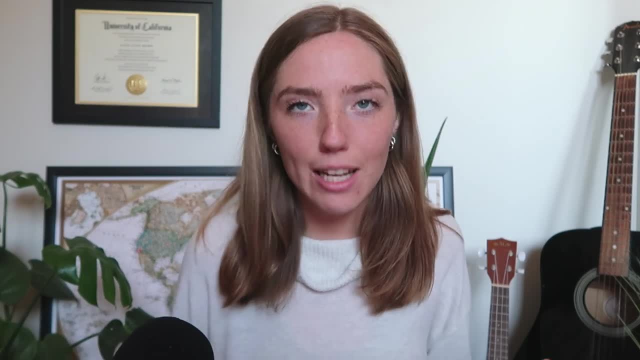 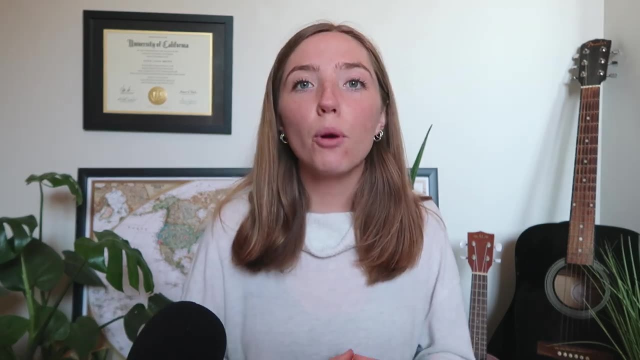 history, biology, language, literally anything human that you can think of. Archaeology is a branch of anthropology. Anthropology has four main subfields. Those subfields are culture, linguistics, biology and anthropology. Archaeology has four main subfields. Those subfields are: 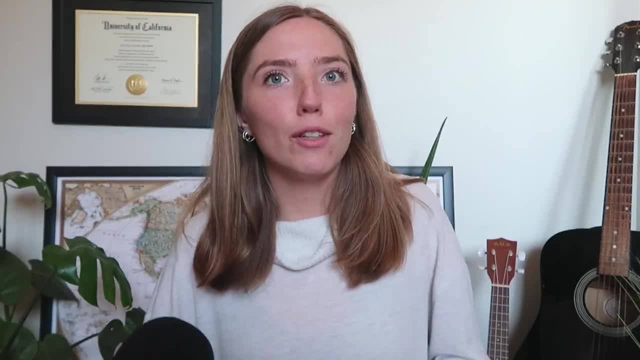 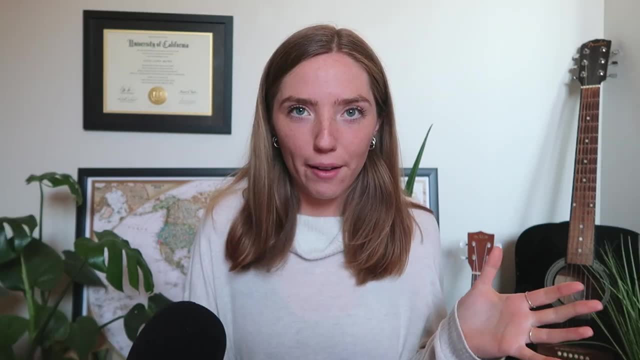 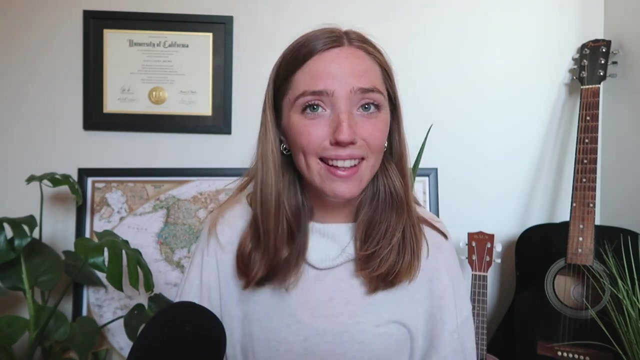 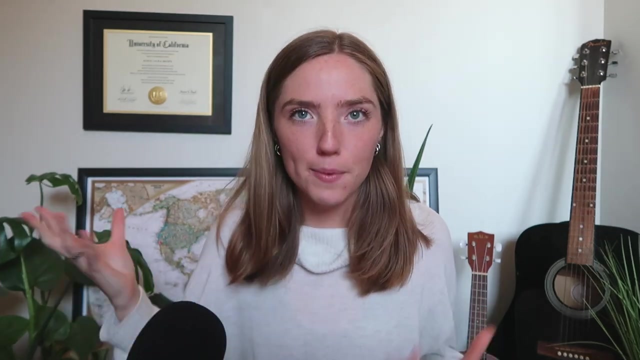 archaeology and archaeology. So, since it's a subfield of a human science, archaeology is understanding humans through excavation. Meanwhile, paleontology has nothing to do with humans. It's understanding basically everything else. that isn't us because, you know, we're self-centered and obsessed with ourselves. So this is all organisms that 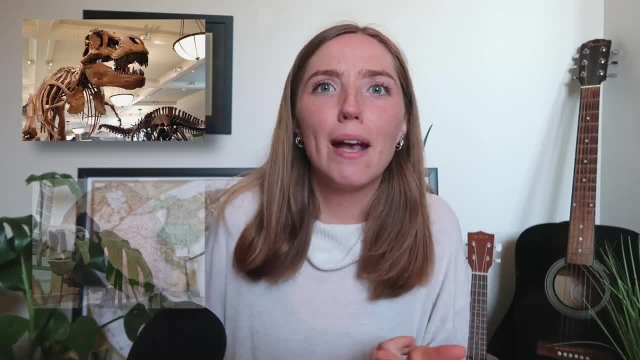 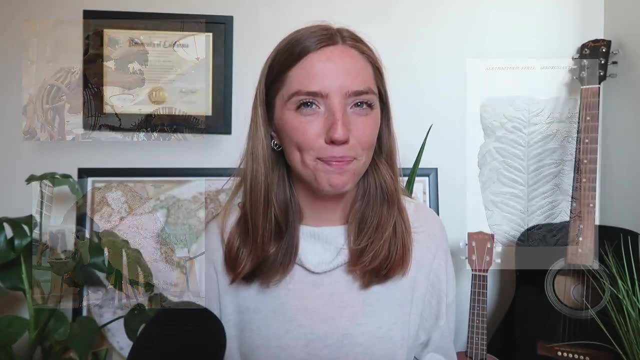 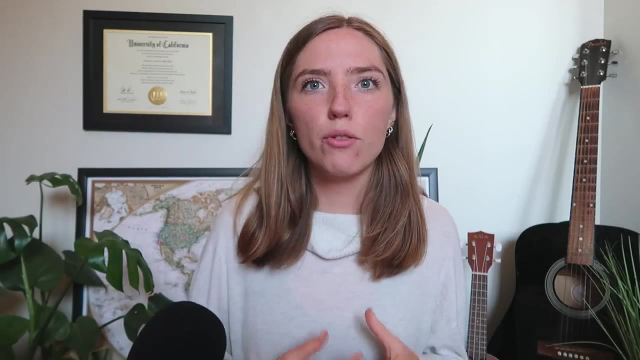 pop up in the fossil record. This is like dinosaurs and megafauna or like ancient plants and stuff like that. That's what paleontologists are more interested in. The next big difference is the kind of remains that these scientists are studying. So archaeologists, when they're going through this archaeological record, they're studying. 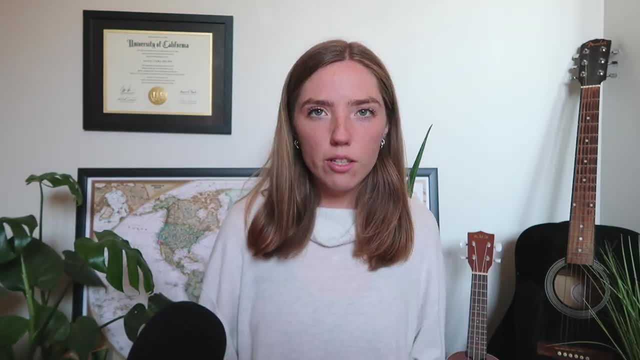 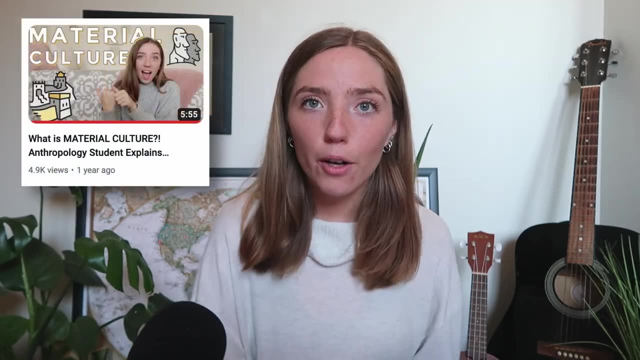 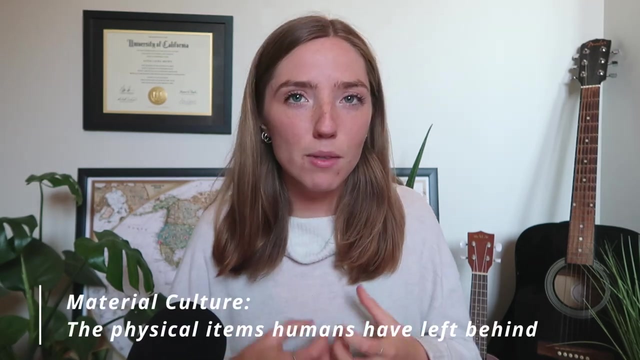 something called material culture. If you're interested in a more extended definition of material culture, I will link a video that I made a while ago on that topic, But the Sparknotes version of it is basically just that material culture are the physical items that humans have. 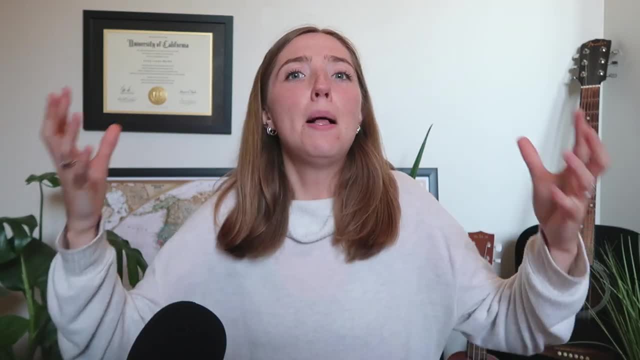 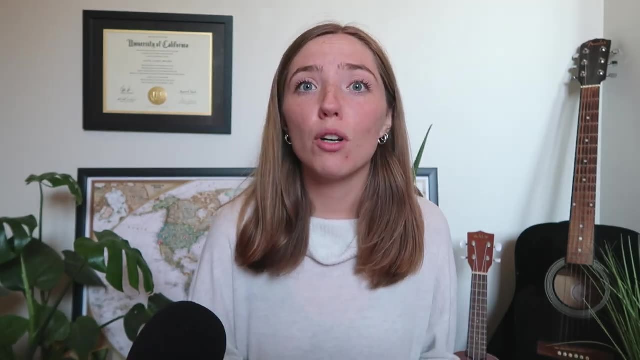 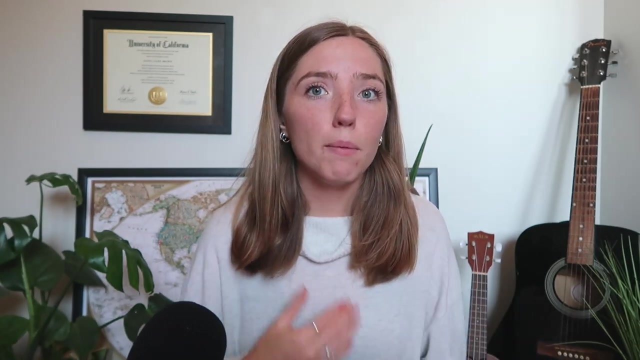 left behind. right We have created giant buildings and homes. We've also created lots of pottery and stone tools, many, many things that do preserve in the archaeological record, And archaeologists call these things that humans have left behind material culture. right, It's culture represented. 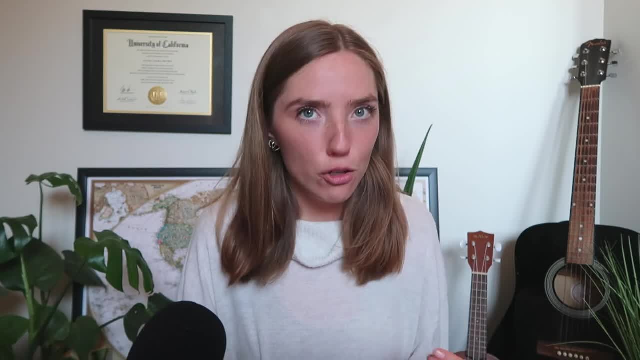 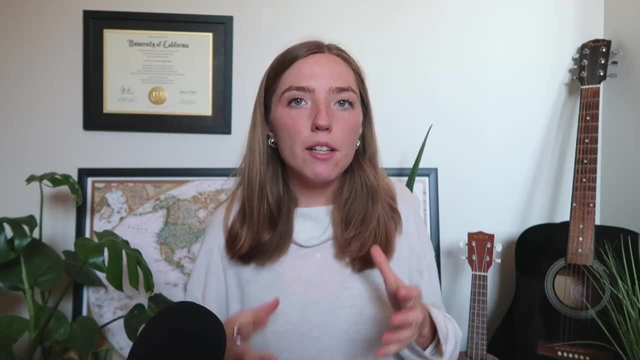 through material Again. go watch that video if you're interested in that. So that's the first thing you're interested. That's what archaeologists are studying. Meanwhile, paleontologists are studying organic material that's been preserved within the fossil record. So if there were, 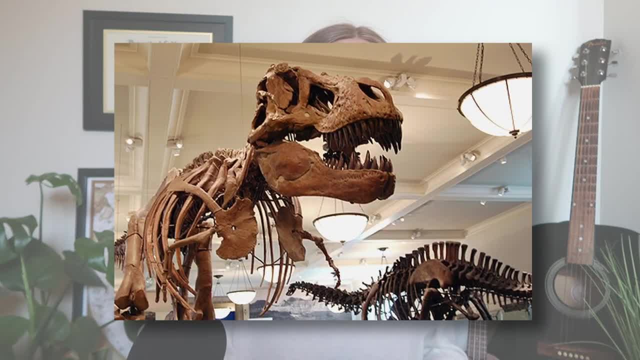 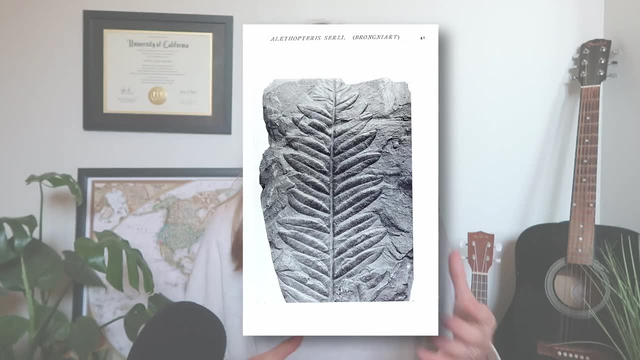 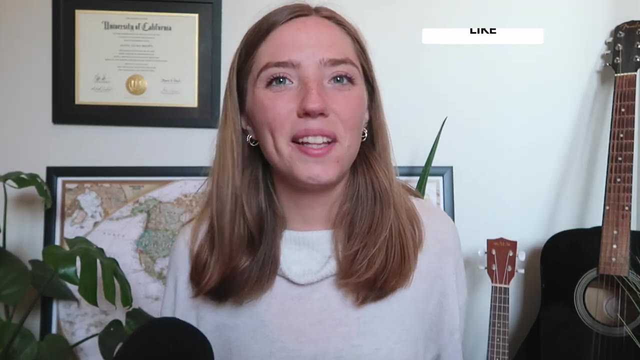 skeletal remains of a dinosaur. that would fall in the realm of paleontology. If there was organic plant matter that somehow preserved in the fossil record, again that falls in paleontology. So yeah, the remains that they're studying are different. Really quickly, if you haven't. 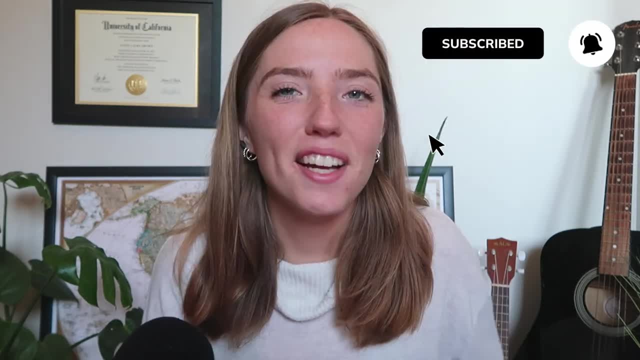 listened to the last episode of the Sparknotes podcast, please do so. If you haven't listened to the last episode of the Sparknotes podcast, please do so. If you haven't liked and subscribed, definitely do that, because I talk about anthropology every single week And we have 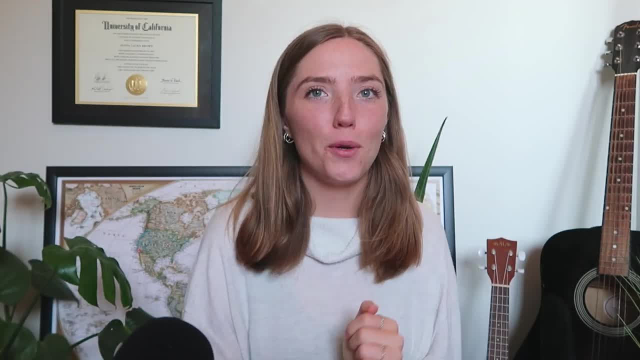 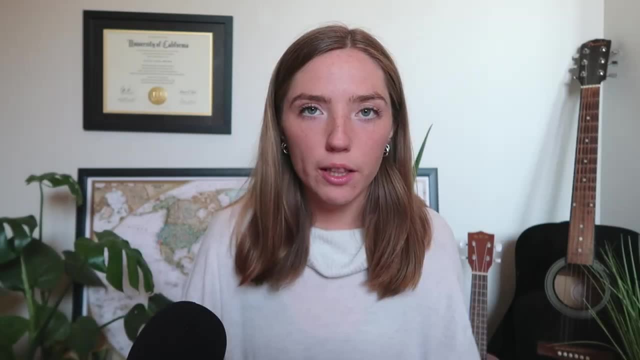 some really exciting things on this channel happening coming soon. So yeah, back to the video. Now we're switching over to similarities. all right, And of course there's a lot of similarities between these two fields, because everyone's mixing them up all the time. I used 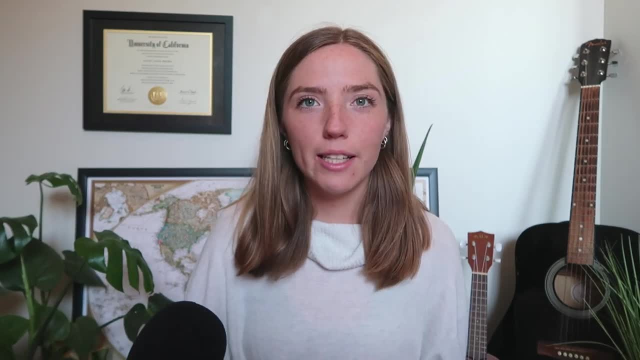 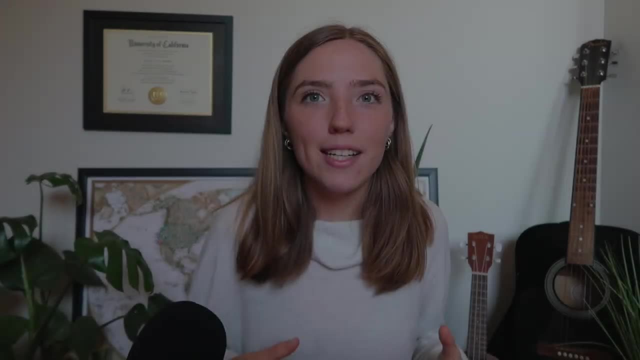 to make this mistake. It's an easy one to make, And one of the biggest similarities between archaeology and paleontology is: we're digging up ancient things right. Both of these kinds of scientists are using the way that the earth has preserved things right. 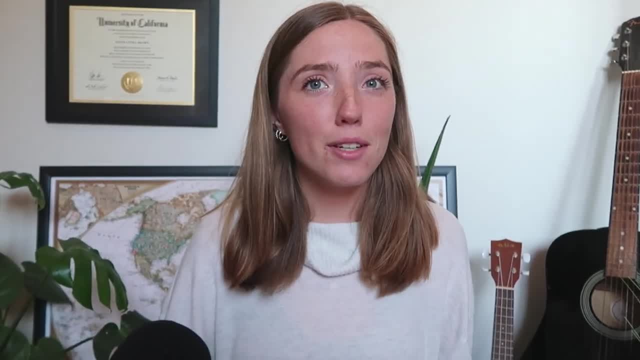 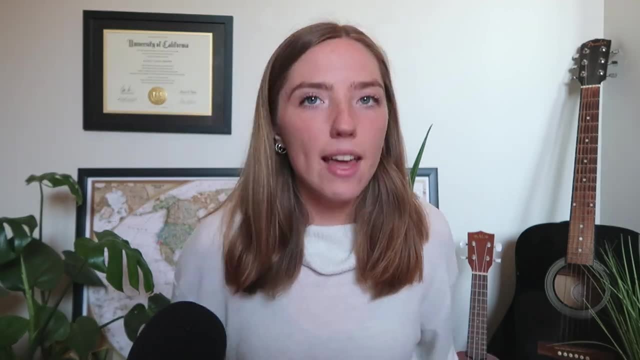 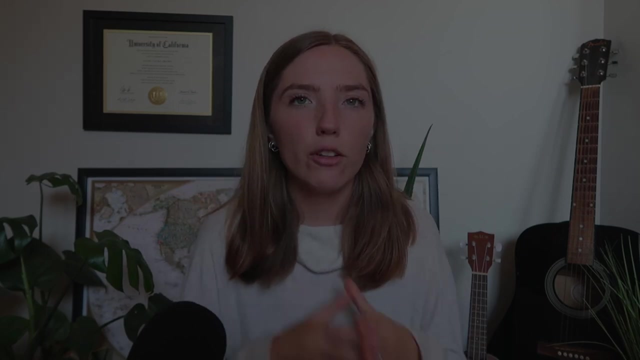 So if you're like, oh, they're just digging stuff up from the ground, Yes, Yes, But it's what they're digging up Again, that varies. Then, finally, there's a lot of overlap in the technology and the scientific method that both paleontologists and archaeologists are using, For example. 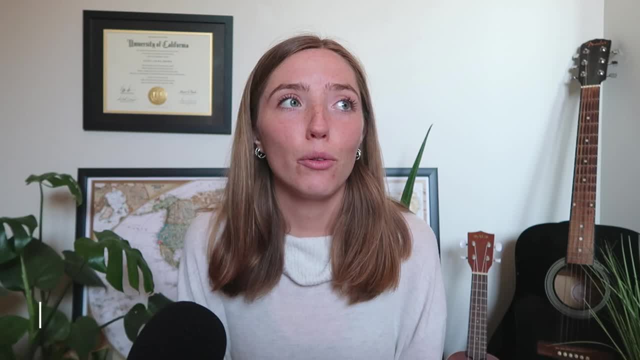 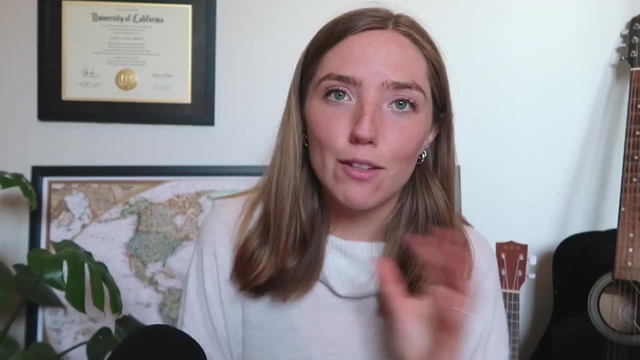 we want to date the things that we have found. This is a done through. I mean a lot of different ways. There's relative dating, absolute dating, Then there's, within each of those kinds of dating, different forms of dating, and all this kinds. 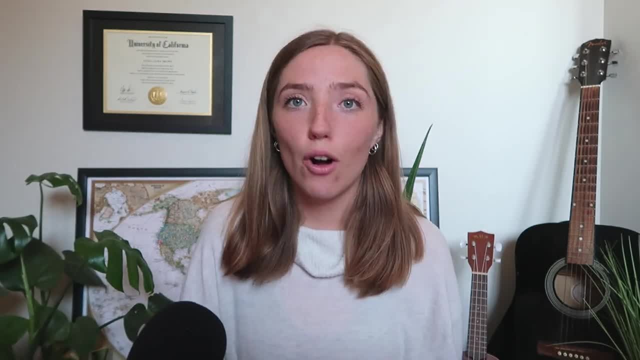 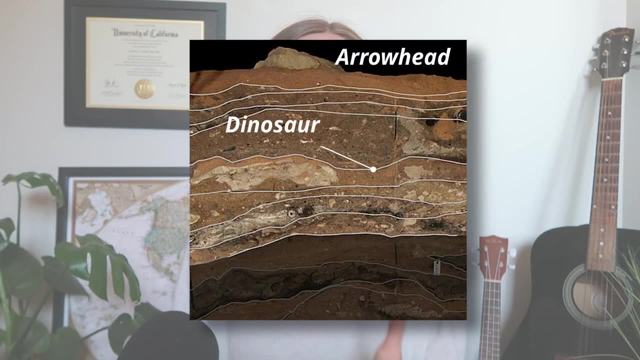 of stuff that both paleontologists and archaeologists are using. For instance, if a dinosaur preserved in between two different rock layers or if an arrowhead preserved within two rock layers, both the paleontologist and an archaeologist might use stratigraphy. 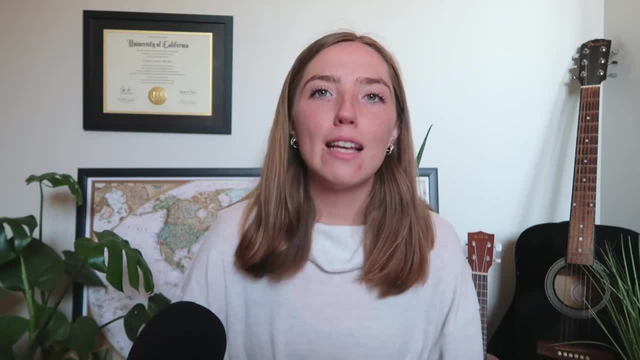 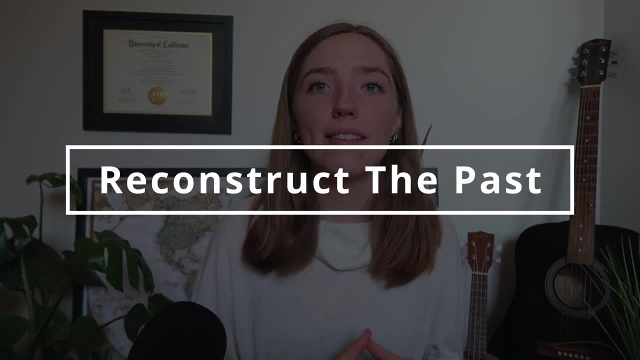 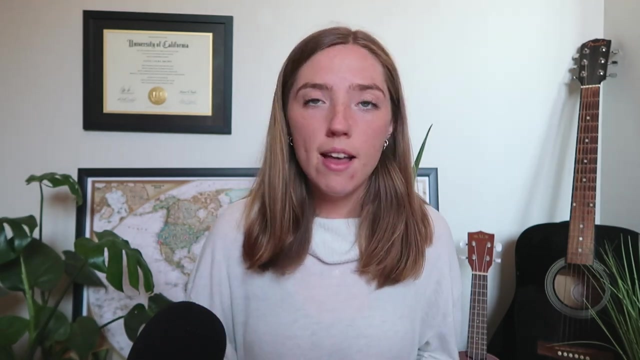 to determine the age. I think you understand. And then, of course, all together, both paleontologists and archaeologists are on this mission to reconstruct the past and understand how the past got us to where we are today. I think, a clear understanding of ancient history, the history of 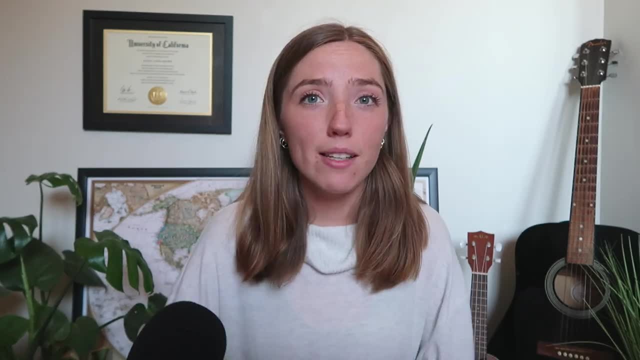 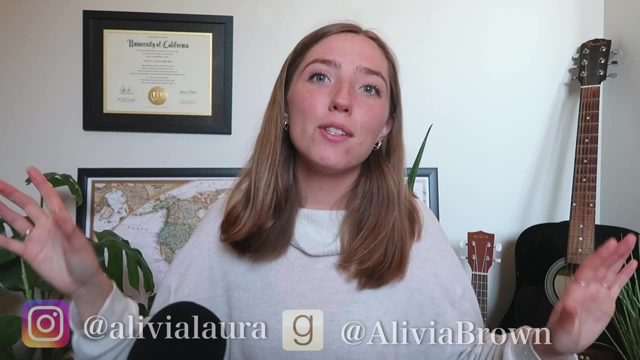 humans, of organisms, of the connection between humans and other organisms. all these kinds of things are very important to both archaeologists and paleontologists. All my sources are going to be linked down below if you're interested in learning more. And yeah, I think that's all I. 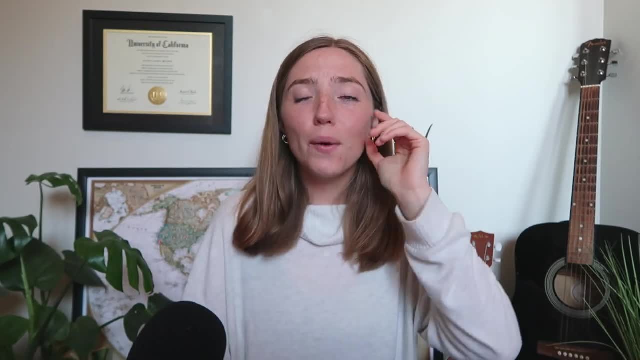 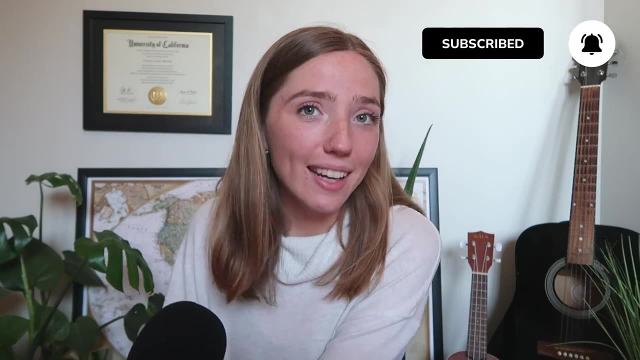 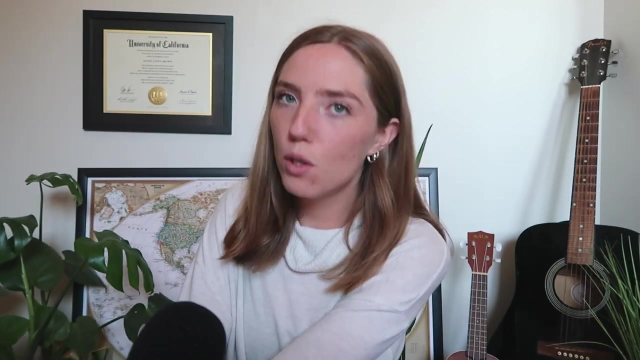 have to say about archaeology and paleontology. But yeah, Oh, also really quick if you're still here. I recently was a guest on the Comfortable Spot podcast with Ken Sweeney. It was a really lovely experience. We talked all about anthropology for 41 minutes straight. So if you want to listen,